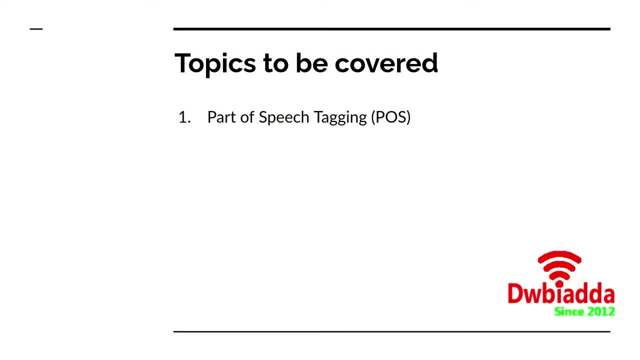 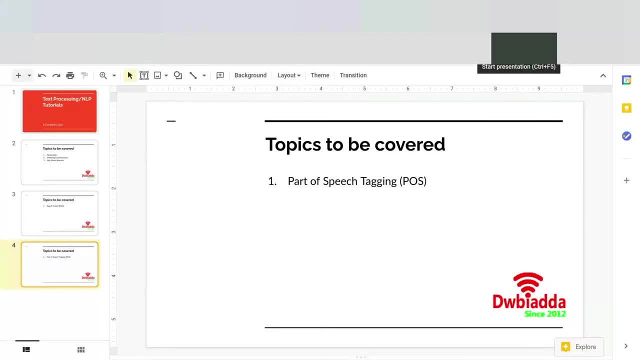 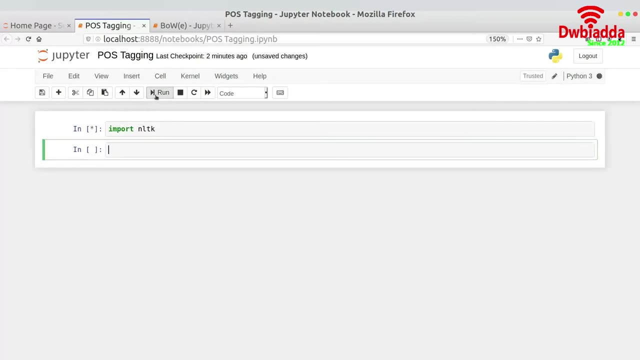 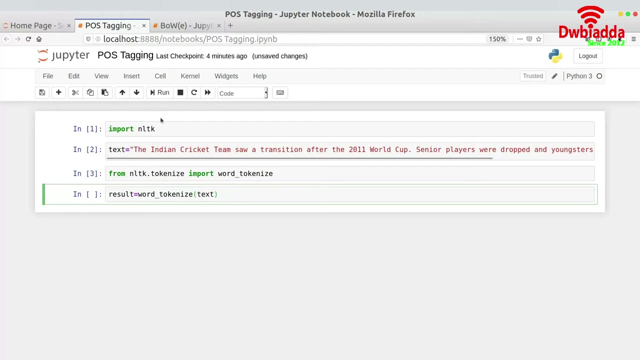 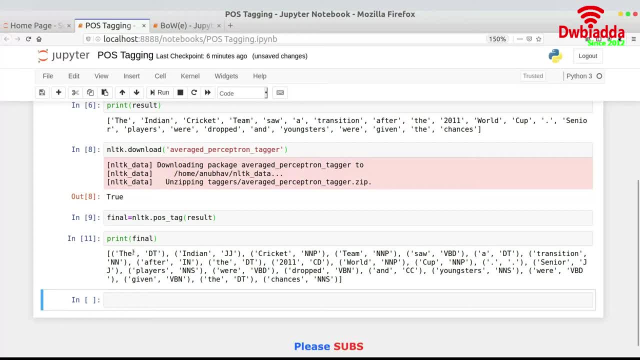 Welcome to DWBI ARDA channel. Please subscribe for latest training videos. Please subscribe for latest training videos. Welcome to DWBI ARDA channel. Please subscribe for latest training videos. Please subscribe for latest training videos. thing that we are getting, but now we do have a fixed tuple over here, uh, and in the tuple the 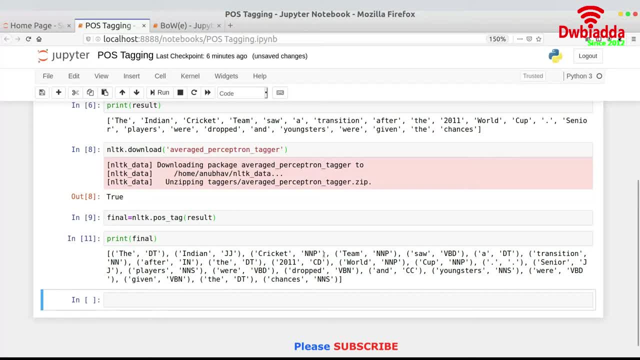 second element is basically something called dt, then jj, then nnp, nnp, vbd, tt and indt, cd, nnp, and we don't know like what, what. this is right, we don't know like what it is trying to represent. so what? i can tell you that, okay, it's trying to represent some, like part of the speech, uh, but we 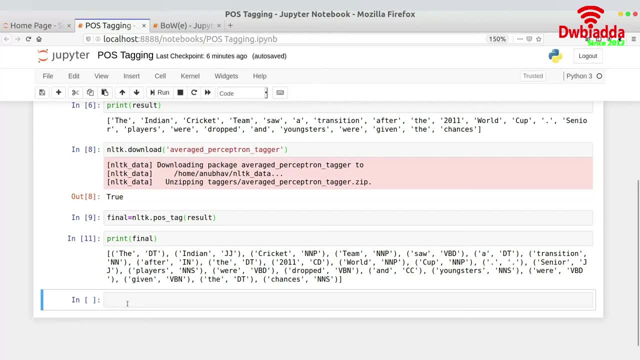 are not sure, like what nnp represents or what jj represents. so for that we do have, like uh, one run in nltk and this is known as nltk, dot, help, dot. i'm not sure what the function is called. i guess this is: you pen set and then i have to pass in, let's say dt. so, uh, the is actually tagged as dt. 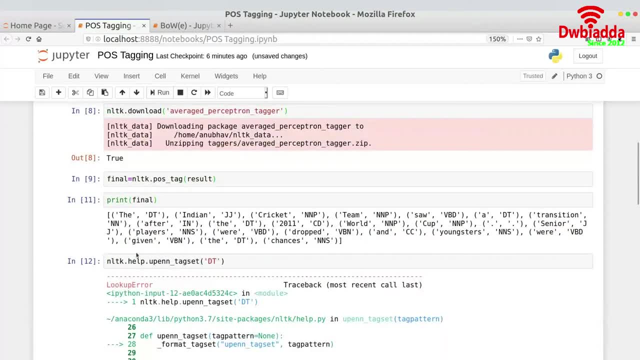 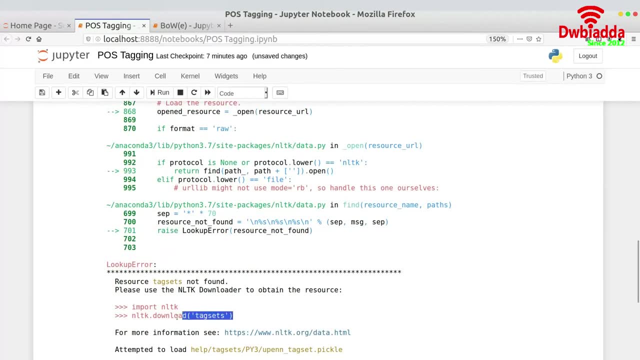 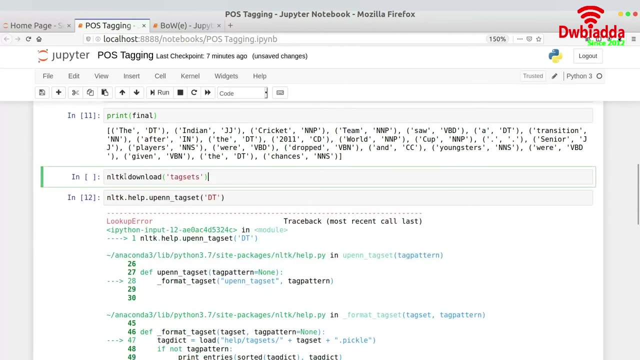 right, so let me just use dt and let me see like what result does it give me? so again, I don't have the required library downloaded as such, so I would have to download this library. so that is why I actually suggested to work on like Google collab kind of thing where you don't have to like download these kind. 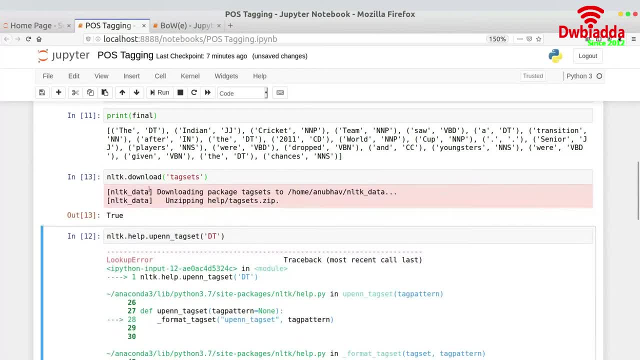 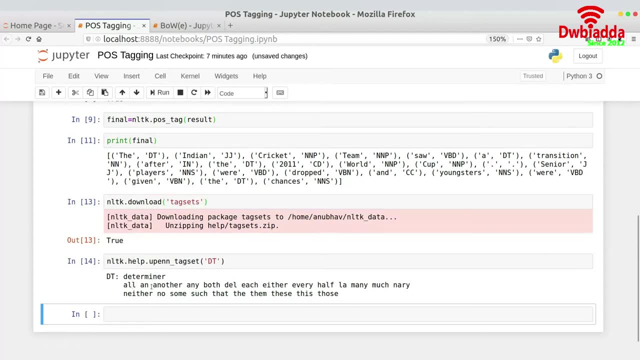 of things because they're already pre-installed over here, but certain you can download this by using the error actually, and you will actually get the result. so, yeah, DT is actually determined, determined and, as you can see, like they have given some examples also, like all and another, any board, then each either. 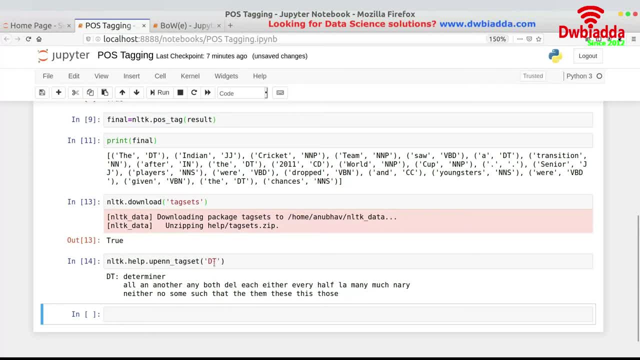 half. all of these are actually a determinist right and like, like the is a determinate determinate itself. and now let us like, look what DJ actually stands for. so I am guessing DJ actually stands for some like something like nationality, but I'm not too sure. let me check its adjective or numerical or 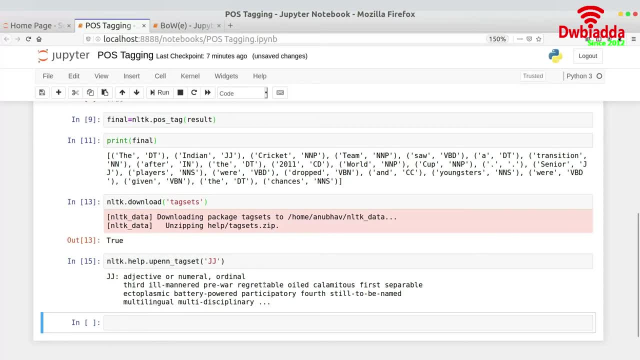 ordinary. there is also, third, ill-mannered, prevaric, creative. okay, so this is the example that is giving us. so it's telling us that. okay, it's adjective, so yes, Indian can be an adjective. and then it's something like NNP, so NNP is. 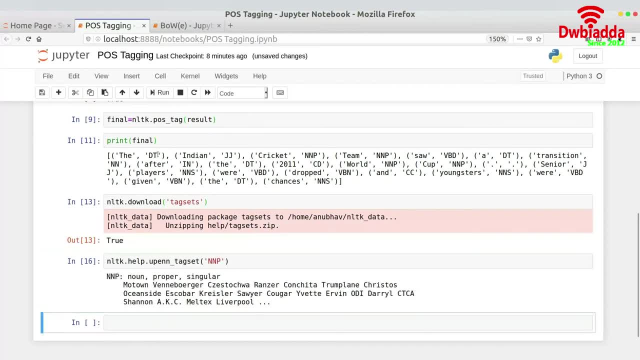 basically, I guess something for now and it's proper now. so cricket is maybe a proper now. I'm not exactly sure if it's a proper noun or not, but yeah, but then you can actually see like it has actually tagged different parts of the speech and able to get different parts right like it can. okay, this is a verb and this is. 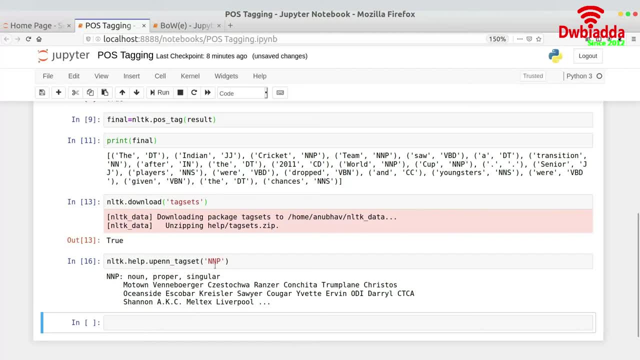 something. so VW, VBD, it can be a verb. so let me check what this is: VBD- and, as you can see, this is a verb in past tense. so yeah, so saw is a verb in past tense, which is absolutely correct. so, as you might have seen, like we can actually get. 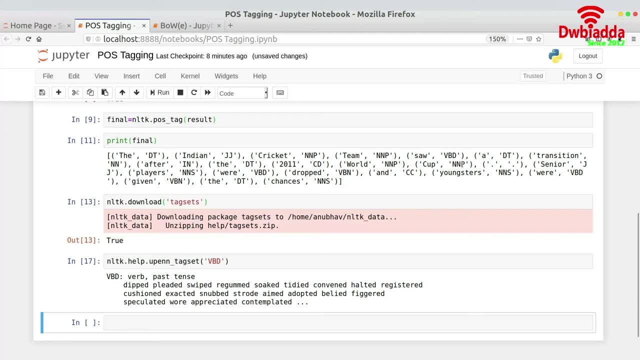 different parts of the speech and all of that kind of thing, using the POS tag thing. but now you should ask me, like, what is the importance? like, why are we actually attacking different parts of this piece so many times? it might happen that by pre-processing you need only some names, right, some proper nouns or 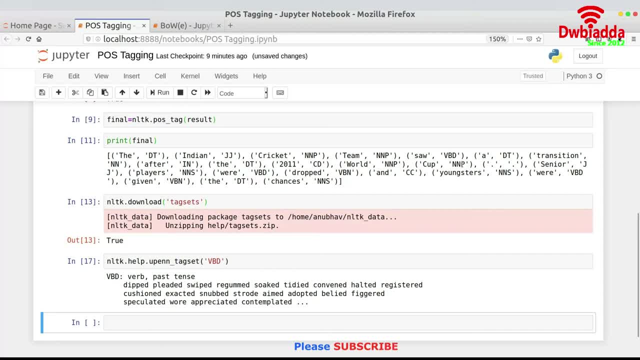 certain verbs only to actually come out, to actually come out right, like I, like you might say, I only require the certain names, or I only require, like, the verb in the speech, or I only require the determinants in the speech and all of that kind of. so this, this will actually help over here to actually separate out. 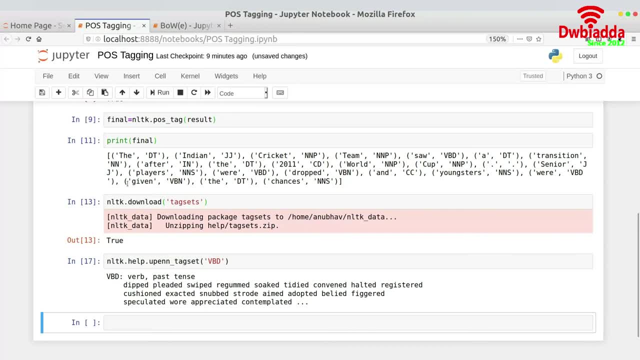 certain parts. so let's suppose I want to get all of the different parts of the speech. so let's suppose I want to get all of the determinants in the speech, like what determinants are basically present in the speech? so it's very easy. I could actually iterate over the final variable.